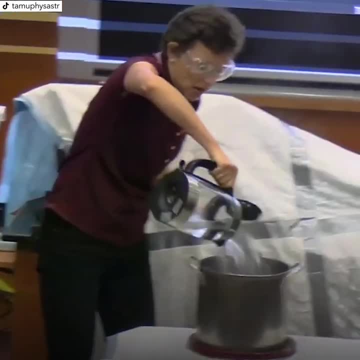 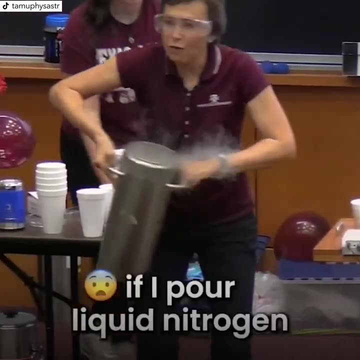 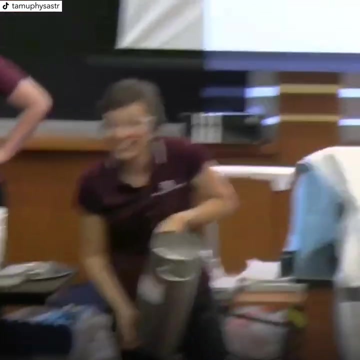 I need boiling water. boiling water, All right, it's hot water. What do you think will happen if I pour liquid nitrogen in this hot water? It's going to go to my throat. Are you ready? Three, two, one. 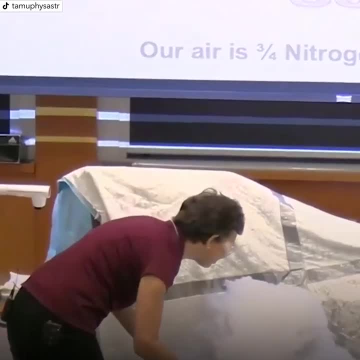 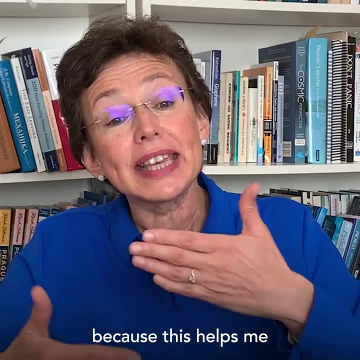 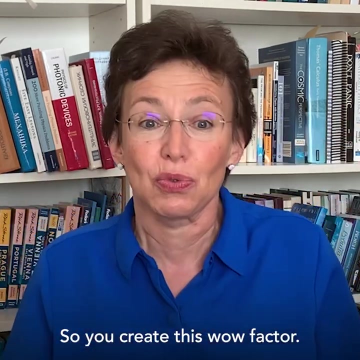 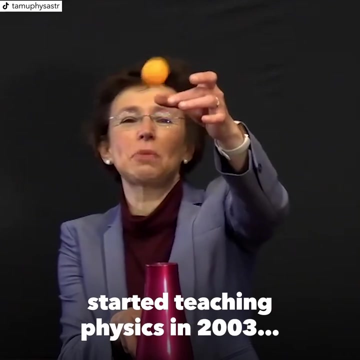 I always bring impressive and impressive physics demonstrations to my first class because this helps me to find this message that resonates with my students. So you create this wow factor. This. look at this, look at this. look at this High speed of airflow. It's not surprising: Airflow pushes it up, but now watch. 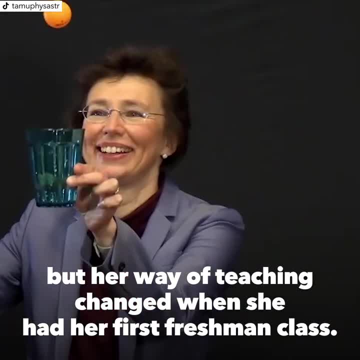 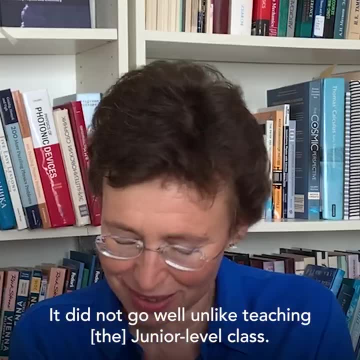 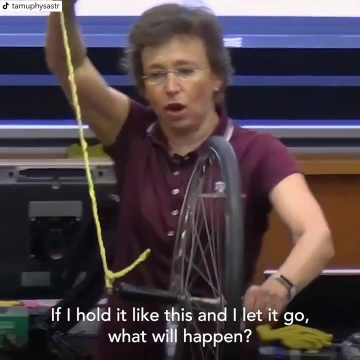 厲害. It was their first class at Texas A&M University at 8 in the morning. It did not go well, Unlike a teaching junior level class. If I hold it like this and let it go, what will happen? It willdrop. 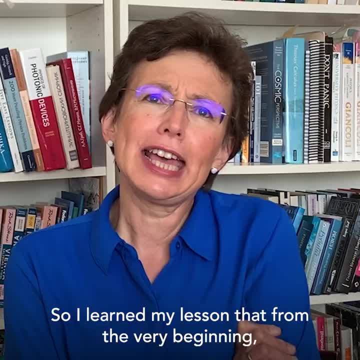 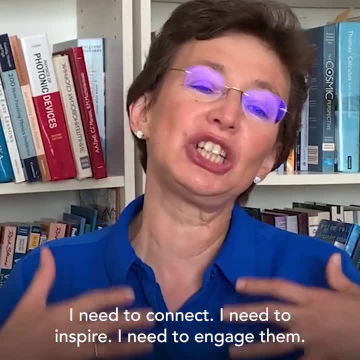 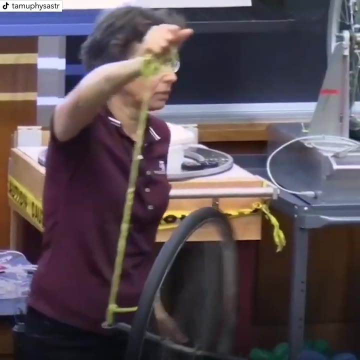 Drop. Why Gravity, Gravity, Boring. So I learned my lesson: that from the very beginning, I need to connect, I need to interact, inspire, I need to engage them. We start spinning it Ready And drop it, And let's face it. 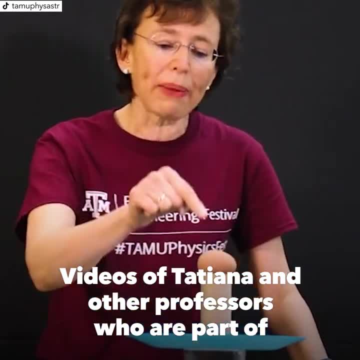 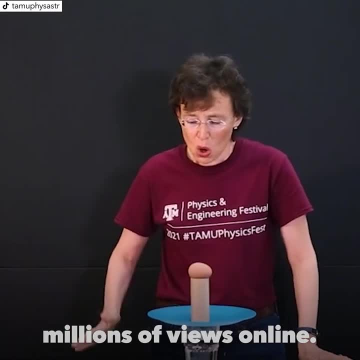 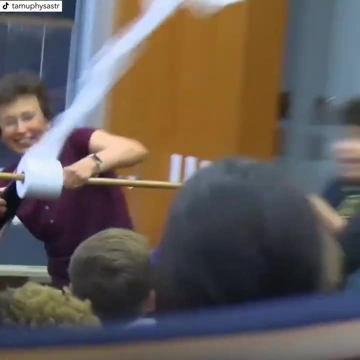 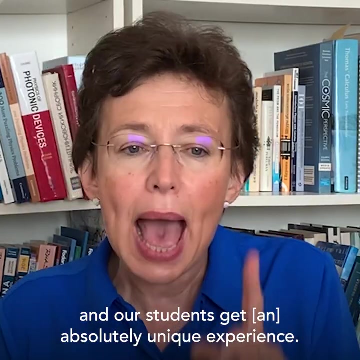 Then the plate will fly, the roller will fly, but the air will not fly. It has inertia, So it will just fall into this glass with water Ready. One, two, three. Let's do it. People enjoy our demonstrations and our students get absolutely unique experience. that is priceless. 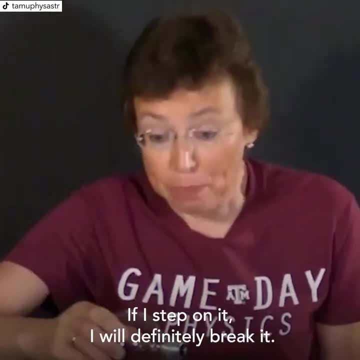 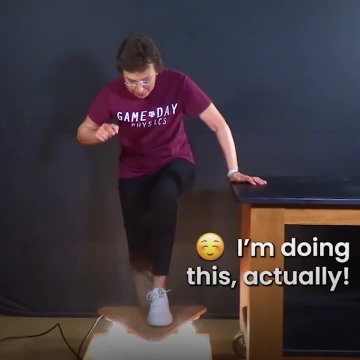 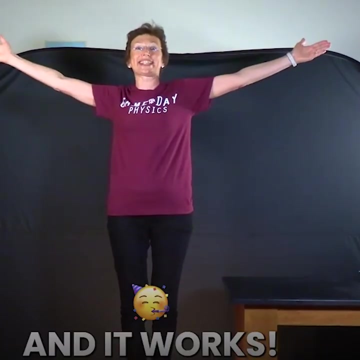 This light bulb is very fragile. If I step on it, I will definitely break it. But what if I have three of them? I will step on them. I'm doing this actually, And it works. One of my favorite things to do is to do this.